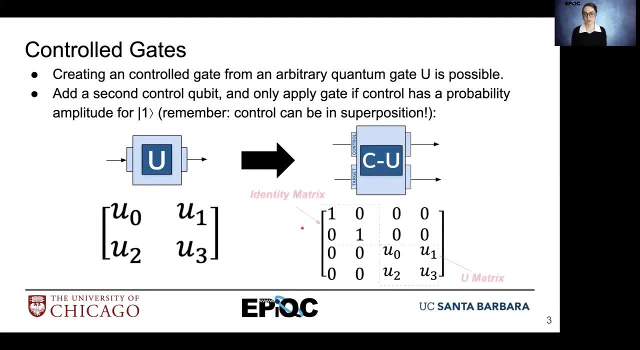 controlled U. Here we can see once again: we have an identity matrix appearing in the top left quadrant and then the U matrix in the bottom right quadrant of the controlled U gate matrix. You can take any single qubit operation and turn it into a controlled operator that uses two qubits. 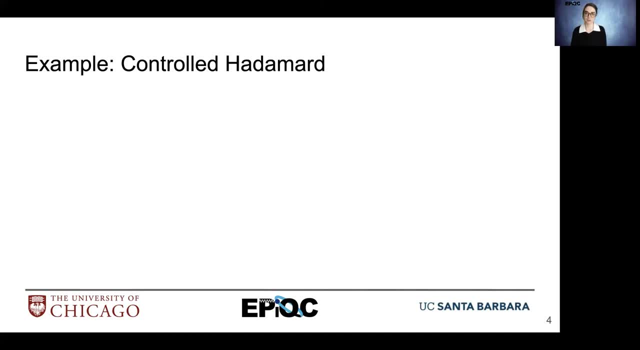 Let's walk through an example. Let's take our superposition gate, our Hadamard gate, and create a controlled variation of that that acts on two qubits. So we have our H gate as a single qubit operation and the corresponding matrix. 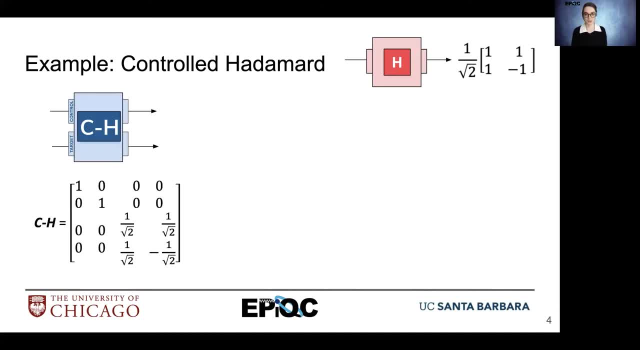 and we're going to form the CH gate or the controlled Hadamard operation. So once again we can note that we have the identity matrix on the top of the matrix on the left, and then bottom right we have our matrix for our single qubit Hadamard operation. 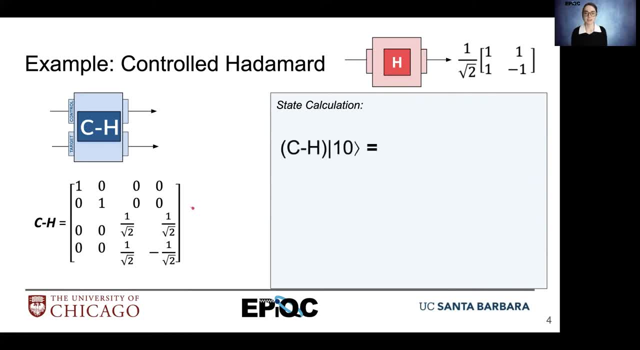 Now let's practice with the state calculation. Let's say we have the state ket 1- 0 that we want to transform by our controlled H gate. So we will have a ket 1 on the top terminal going through the control input, a ket 0 going through the target terminal. 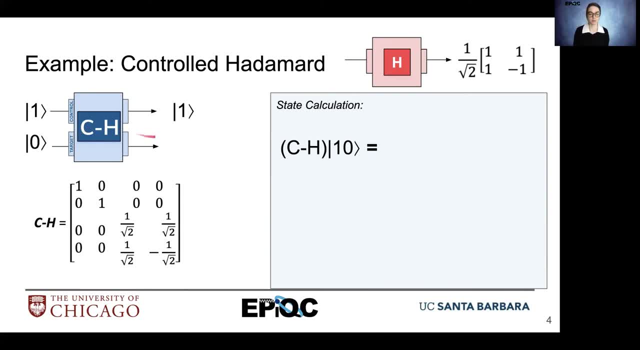 the ket 1 will pass through the top, and then our ket 0 will pass through the top, and then our ket 0 will pass through the top. 0 will be transformed into a state of superpositions. We have 1 over square root of 2. 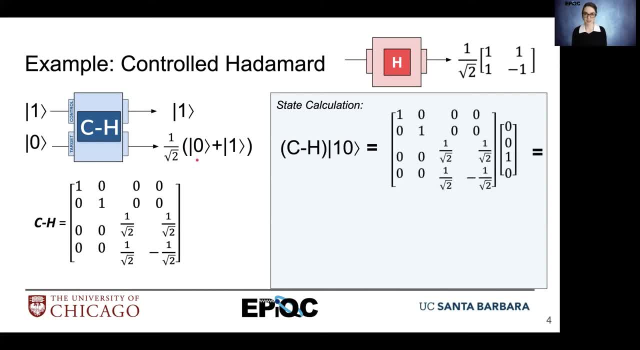 multiplied by ket 0 plus ket 1.. Let's validate that with a matrix multiplication. So we have our matrix for our operation. Then we're going to multiply that by our vector. that represents ket 1, 0. And if we take our results, that we predicted, so ket 1, tensor 1, square root of 2. 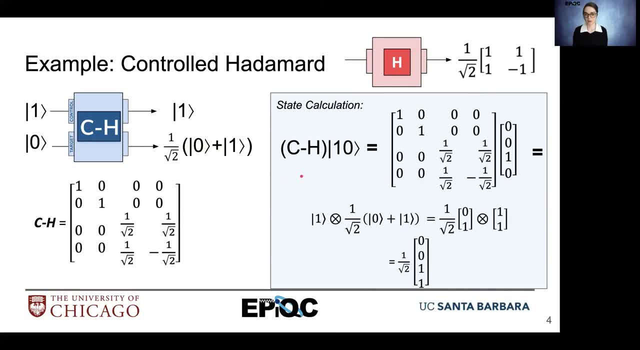 times ket 0 plus ket 1, we can write that in our bra ket notation, write it in our vector notation. take the tensor of that and we get our final result. And that's what we anticipate whenever we do our matrix multiplication. So what we predicted as our output matches the result of our 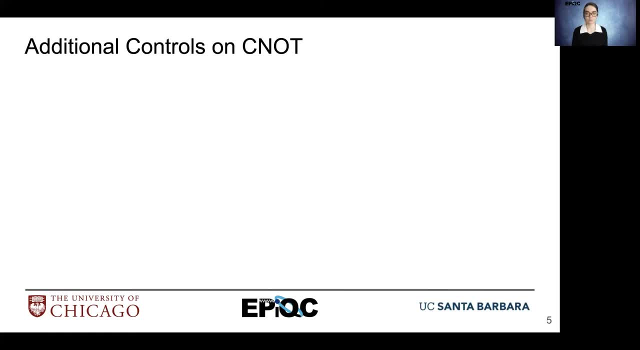 matrix vector multiplication for our final state. What happens if we add additional controls to c0?? So that would be our matrix multiplication And then we get our final result. So that would be the controlled c0 or the cc0 operation, which is also called the Toffoli gate. So the Toffoli gate. 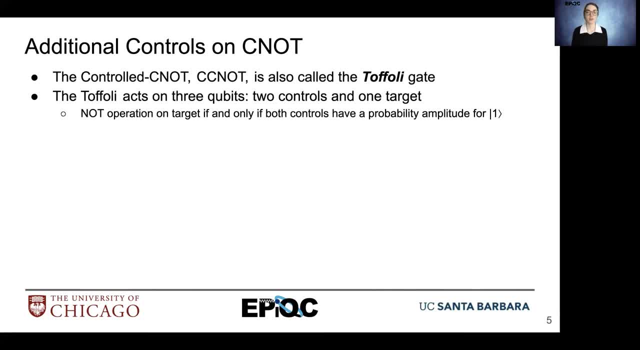 acts on three qubits, two controls and one target. The not gate operates on the target if, and only if, both controls have a probability amplitude for one, Because, remember once again, our controls can be in a state of superposition, So they may not 100% be in the state of ket 1.. So here we have. 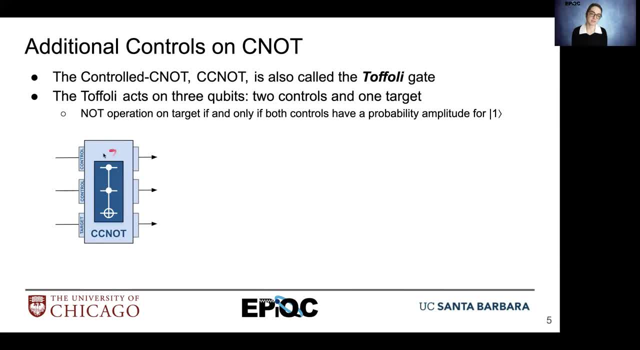 our cc0 gate or our Toffoli gate. This is the symbol that you'll often see in schematics or circuit diagrams for quantum circuits. We have two controls and then a target, so three total qubits that we're acting on, And here is the corresponding matrix. If we look at 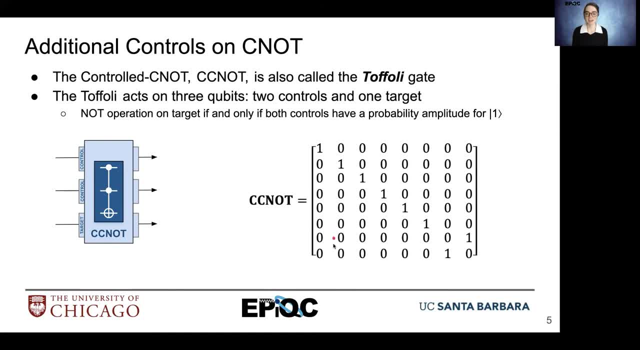 the dimensions of this matrix, we will see that it's an eight by eight matrix, And that makes sense because we have two to the three, which is equal to eight, and we're acting on three qubits. So our final matrix that we use to represent that operation is going to be eight by eight. 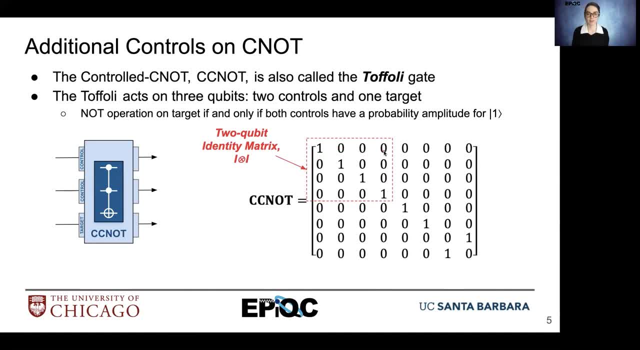 If we look at the top left quadrant, that is the two qubit identity matrix or I, tensor I, and then the bottom quadrant is our c0 matrix. So we just took our c0 matrix and added a control and we followed basically the same procedure that we did for taking a single. 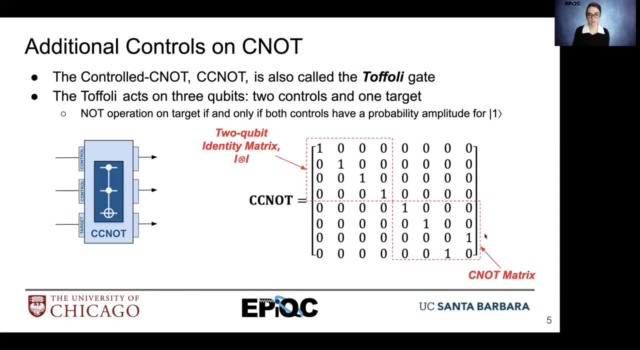 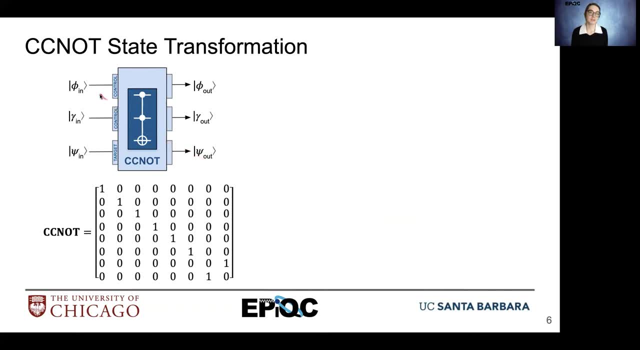 cube operation and adding a control line on that. Let's examine what happens with states when we transform them by the cc0 gate or the Toffoli gate. So we have phi, gamma and psi as our input quantum state, and then we also have their outputs as well. So we have our following matrix: 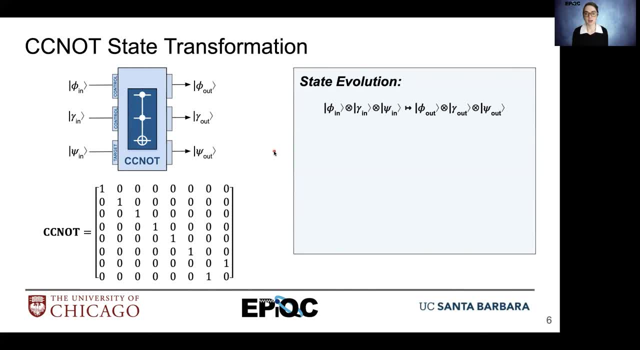 and when we do our state evolution, we will see that our transformation from input to output will be very similar to the CNOT gate, but we now have an extra control we have to take into consideration. So if we look at our state evolution, we're going to see that our states